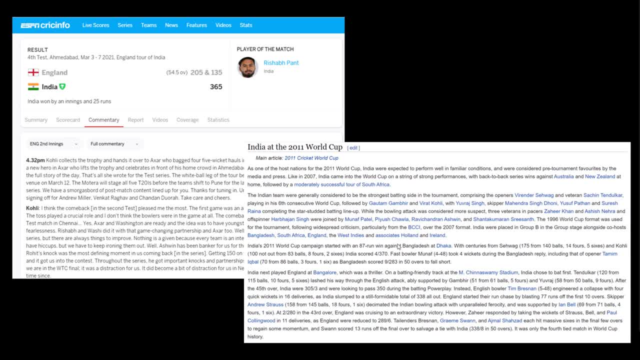 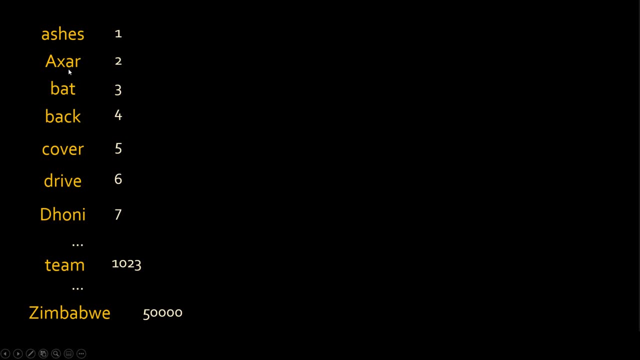 Wikipedia and so on. You try to grab all the articles to build your language model and you build a vocabulary out of it. So vocabulary is nothing but list of words. So let's say this is your vocabulary. You start withurt1.. 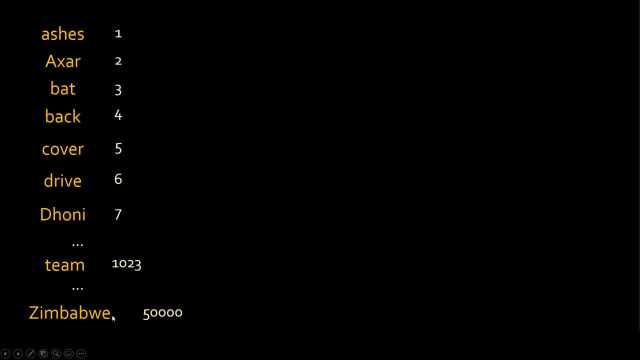 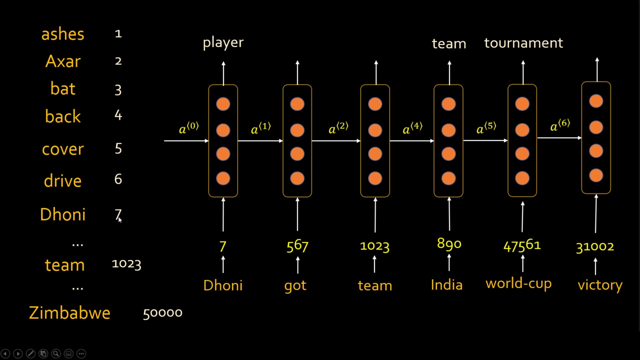 is the name of the player, Dhoni is the name of the player, Zimbabwe is the name of the team, and so on. Let's say my vocabulary has 50,000 words. You can assign unique number to each of these words and then you can use those numbers as an input to your RNN. For example, Dhoni has number 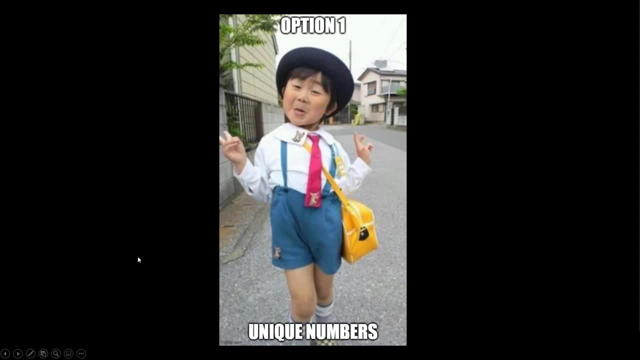 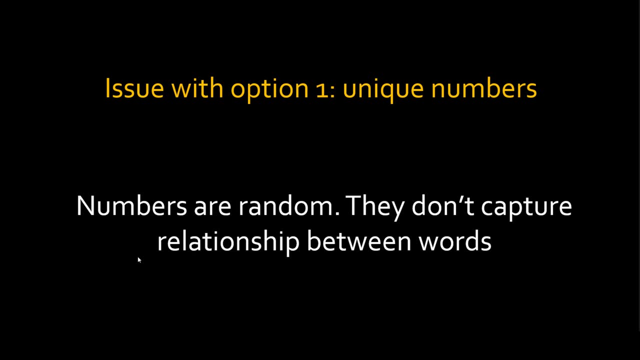 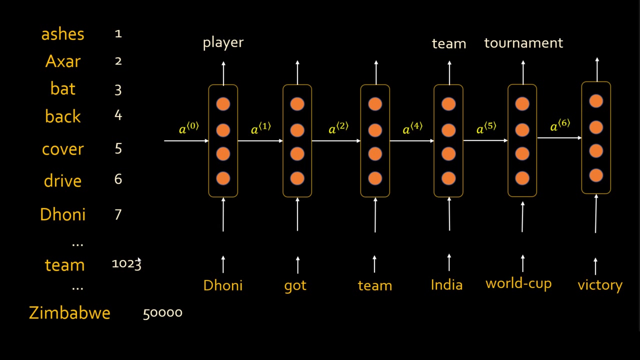 seven, so see use seven here. Now that's your option number one, basically converting words into unique numbers based on your vocabulary. but there are issues, such as the numbers are random. they don't capture the relationship between two words. For example, in this particular case, Dhoni's number is seven, Akshar's number is two. Dhoni and Akshar, both are players, so maybe these: 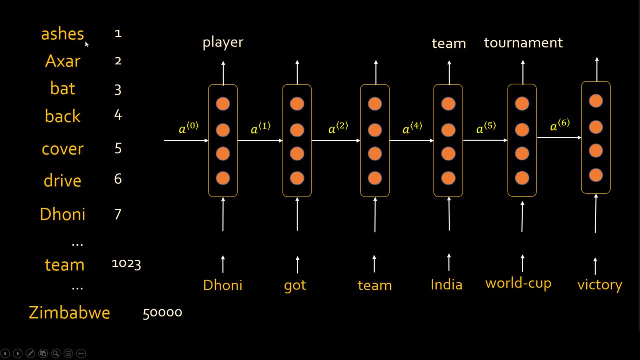 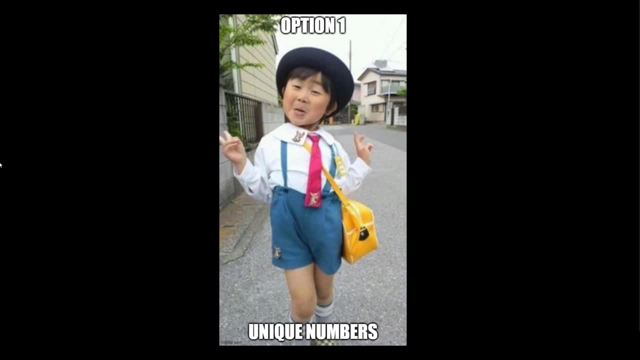 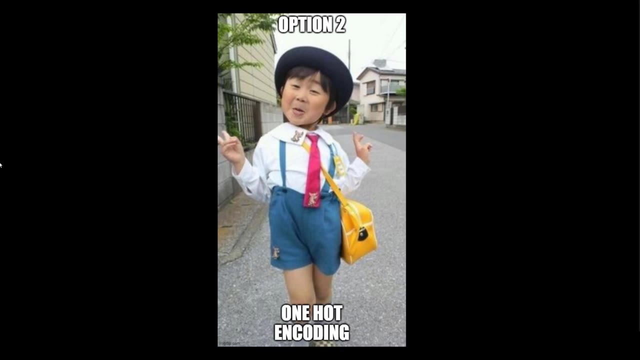 numbers should be similar, but they are far apart, whereas Asish is the name of the Toonam and it is more near to Akshar. So these kind of random numberings cannot capture the similarities between the words. So then, the second option you have is one hot encoding. If you have seen my machine learning videos, you might have seen one. 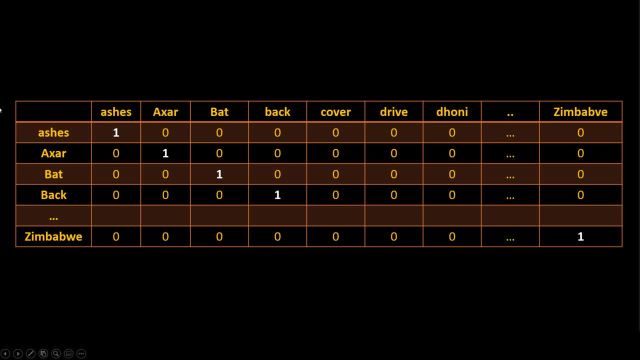 hot encoding tutorial, which is basically you take all your words and when it is Asish for Asish, you put one remaining words, you put zero and you get a vector. For example, the vector for Akshar would be 0, 1, 1.. So wherever Akshar appears, you put one remaining numbers are zero. So this is a very 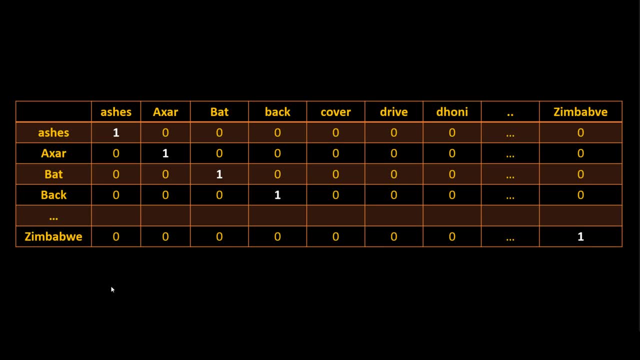 popular approach in machine learning. If you have a machine learning video you might have seen one machine learning. but this also have a couple of issues, like number one issue is obviously they don't capture the relationship because, see again, there is no relationship established. you know if 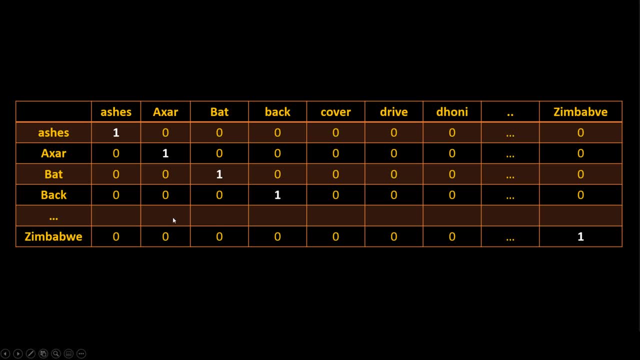 you are if I don't tell you the words, if you are just looking at these numbers, you can't tell if two words are same. you know, like banana and grapes, for example, these are the two fruits. So if you have these two fruits, maybe you want their vectors to be a little similar. 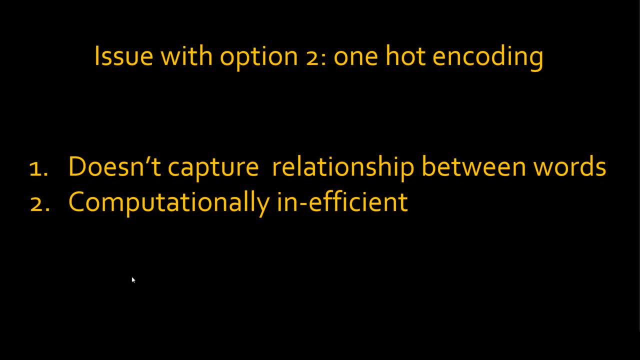 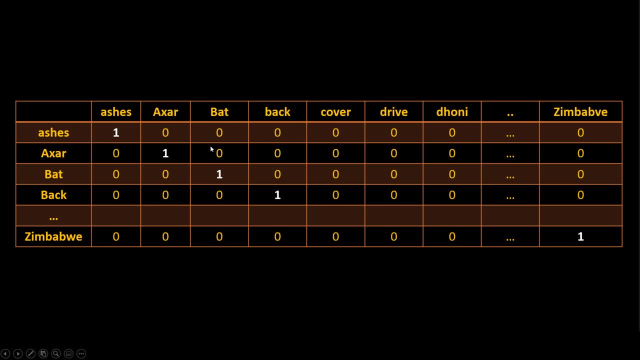 The second problem is it is computationally inefficient. If your vocabulary has 50,000 words, for each word you get a vector whose size is 50,000.. Often in machine learning problems, the number of words could be in millions or trillions, millions of billions, not, maybe not trillion or it. 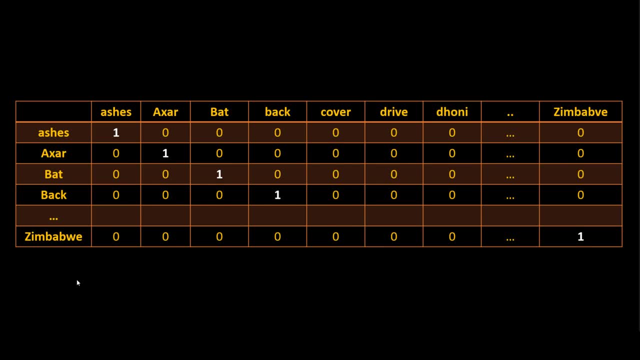 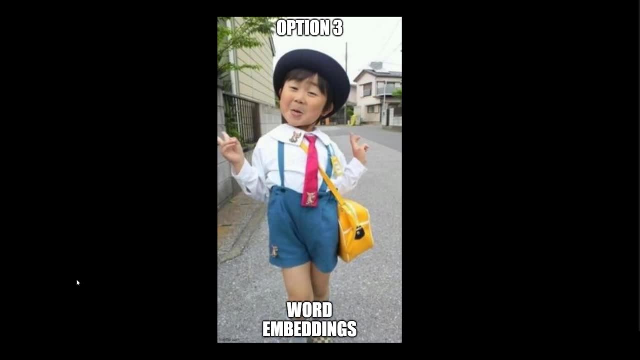 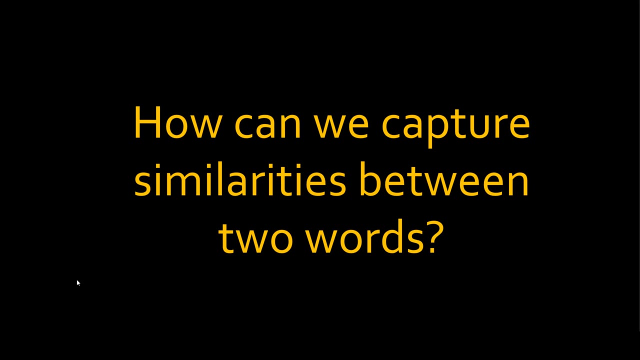 could be trillion in future, but you get the point. So the computational cost is very, very high. So the third option you have is using word embeddings. Word embeddings allow you to capture relationship between the two words. Let's see how do you capture similarities between two words. So 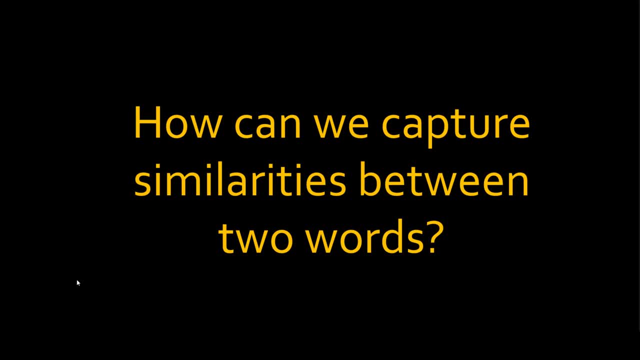 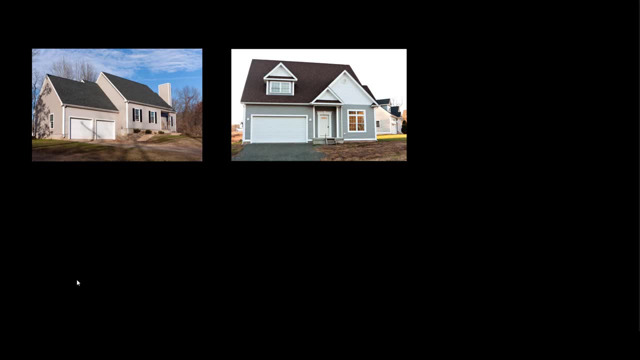 let's take the example In order to explain how word embedding work. I want to take you back to your first machine learning problem, which is predicting home prices. So if you have two homes and you want to, let's say, figure out if the home prices are going to be higher or lower, then you 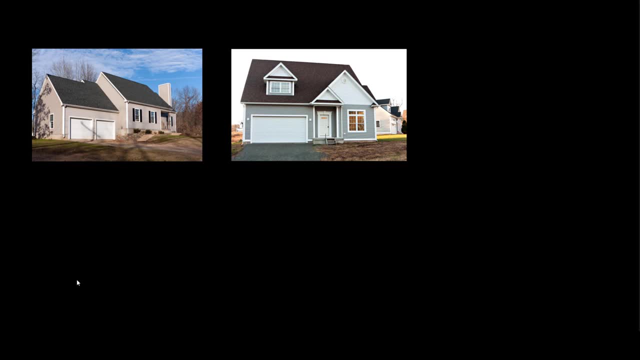 can use word embeddings. So if you have two homes and you want to, let's say, figure out if these homes are similar or not, How can you do that? Well, you look at the features of the home. What are the features? It's simple, right, like the bedrooms area, bathrooms and so on. So if you 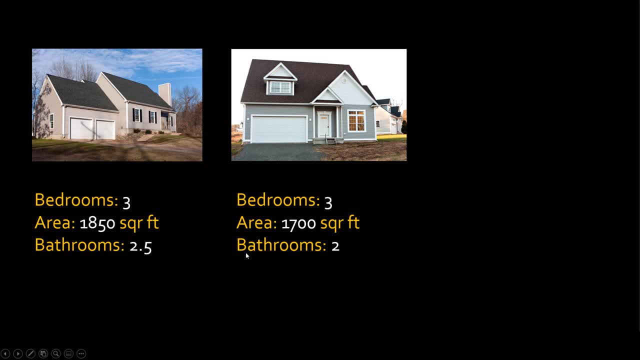 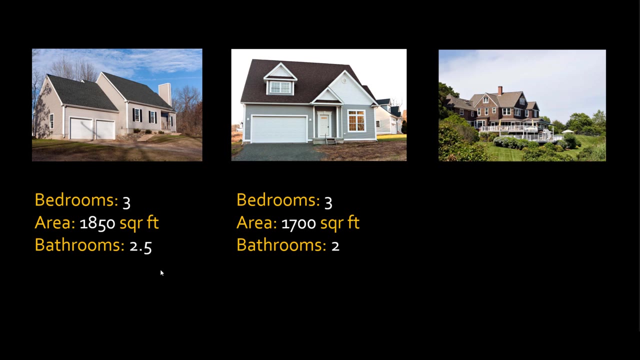 look at these two homes. the bedrooms are same, area is almost same, you know, 7800 versus 1850.. Bathrooms are also kind of near to each other. So then we can say that these two homes are similar in terms of features. If I have a third home, let's say big mansion, you know which is very big home. 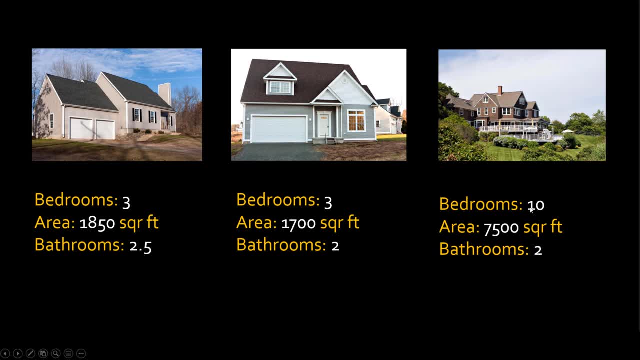 and if I look at the features of this home- you know the feature vector would be 10, 7500 and 2- and when I compare this vector with this vector, I will obviously figure out that these two homes are not similar. Can we apply similar concepts to? 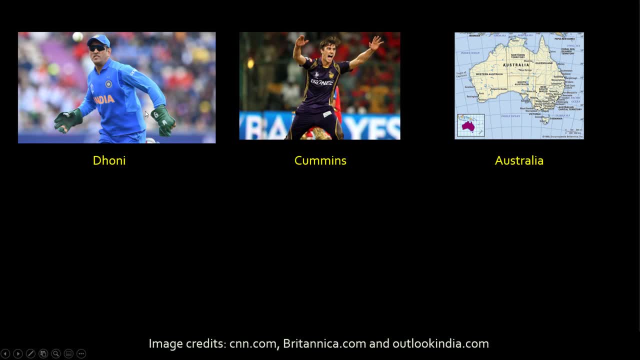 the words. Let's say these are my words- Dhoni Cummins. I put just pictures for the reference. we are comparing just the words. okay, so Dhoni Cummins, who is an Australian player, and Australia, which is name of the country, How can you compare these three words? now, as a human, we know that. 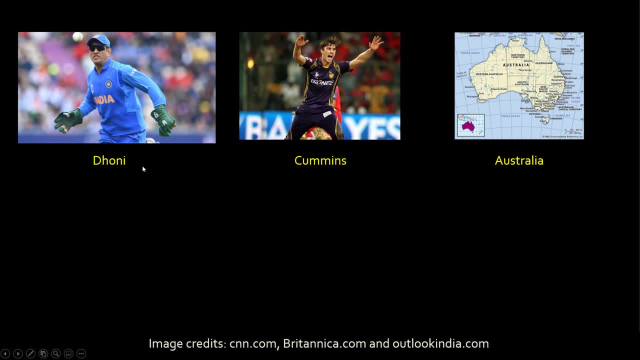 Dhoni and Cummins are similar because these are players- you know name of players- but Australia is not similar because it's the name of the country or name of the team. So then just think about: is there a way to retrieve the words that are similar to the name of the country? 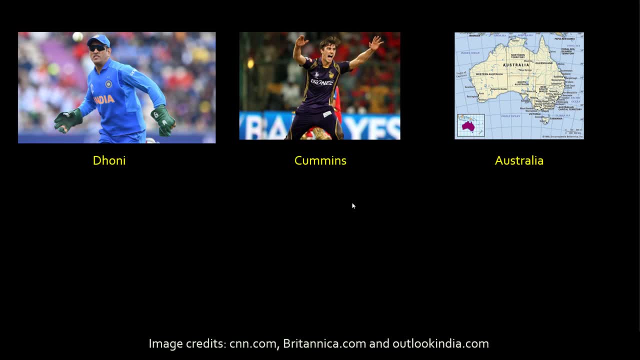 You can retrieve features from these words. if you think hard, you might be able to come up with some features, such as person, whether the person is healthy or fit. location has two eyes, has two, government has government. so in the case of Dhoni, he's a person, healthy, fit. yeah, he's pretty healthy. 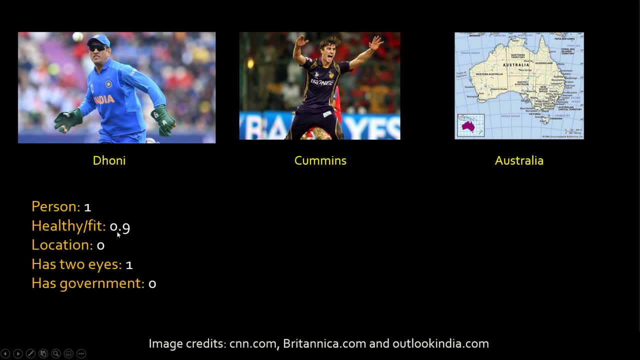 but you know, maybe 0.9 we can put some number. one means like perfect, 0.9 is like really healthy. is Dhoni a location? Well, no, so 0. does he have two eyes now in order to qualify for the? you know international cricket. 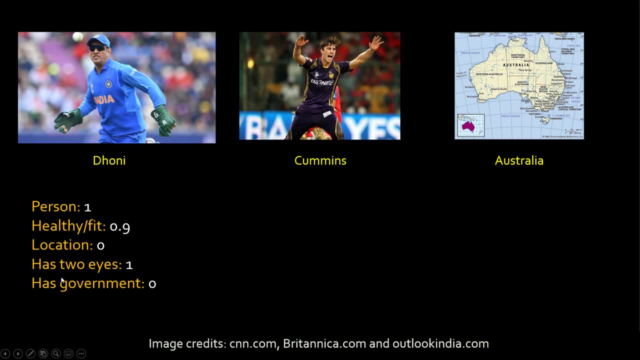 you need to have two eyes, so that's why I'm so. there could be many features. I just handcrafted these features. there could be 10 features here. you know how fast he can run. whatever then has government. does Dhoni have government? no, that doesn't sound. that sounds weird actually. 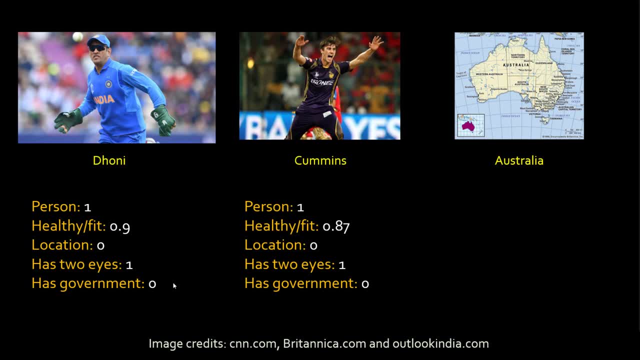 so then I put zero and when I put similar numbers for Cummins I will probably get similar kind of vector. you know, here I have 1.9010, 1.87010 kind of similar vector and and I put these numbers randomly, okay, so there's no logic to it. so don't tell me like. 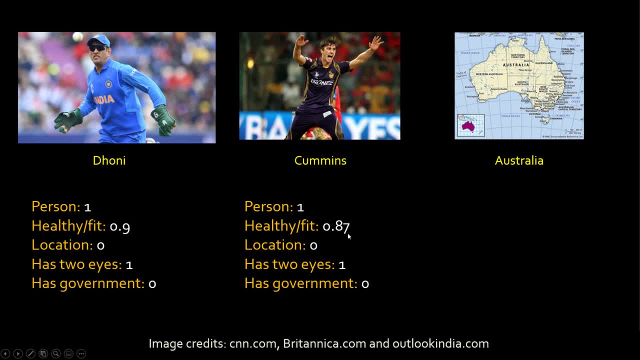 don't ask me how the number for Cummins is 0.87 here, but for Australia, when you put the same number. Australia is not a person, so of course zero. but he often has a location, so it's one. Australia has government, so it's one. 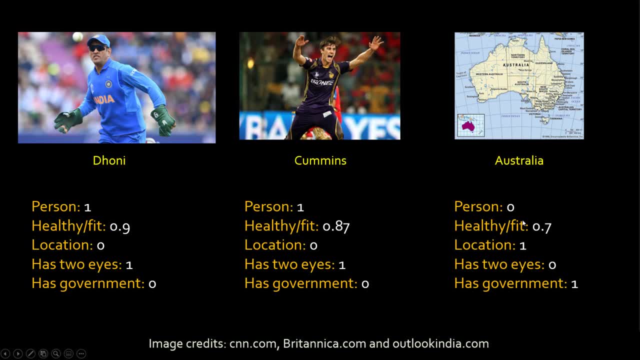 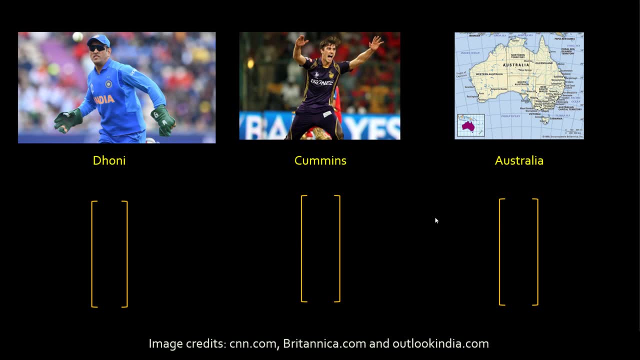 And if you have any other countries, they will match the feature vector that I have presented here. so essentially what we did is we converted word into a vector. vector is just a bunch of numbers, right, and when I converted that what I found is Dhoni and Cummins are kind of similar. 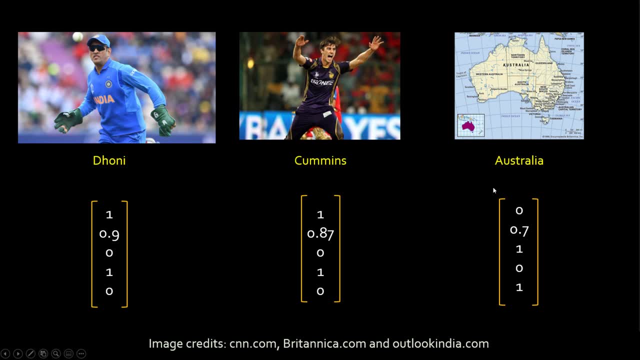 see 1.1.9.87. and. but Cummins and Australia are not similar, or Dhoni and Australia are not similar because see 1.0.9.7. yeah, of course 0.9.7. why 0.9? oh yeah, maybe healthy and fit meaning for a. 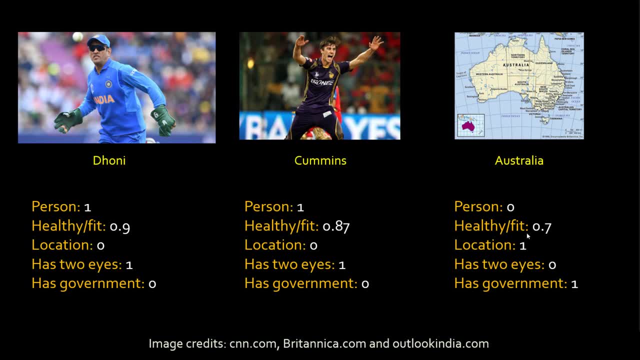 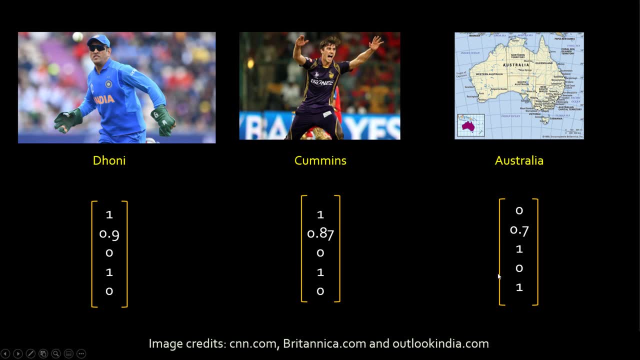 country is if the country is healthy economically. Australia is doing pretty good, so we can say 0.7. yeah, so some of the numbers might match, but the entire vector, if you compare the similarity, it is not very similar. so now we found this feature feature vector for the word. 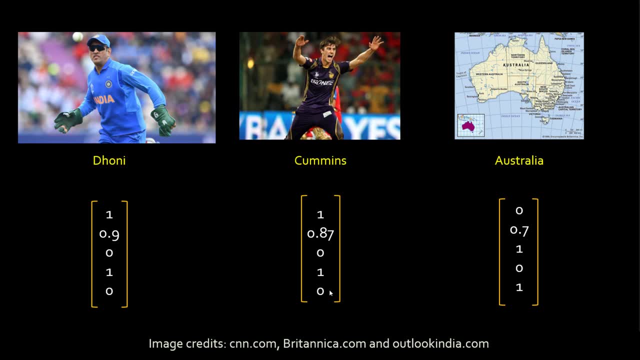 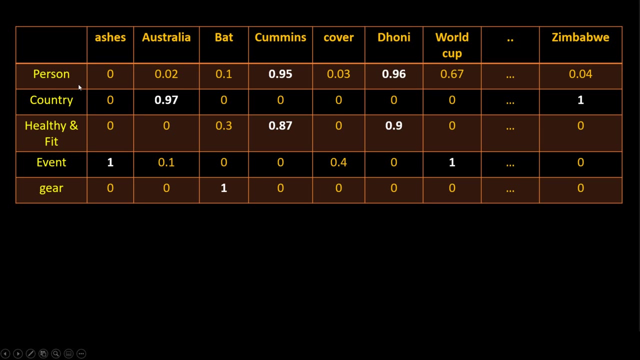 and that could be very effective to solve a variety of problems in NLP tasks. and this is basically word embedding. so if I look at our original vocabulary, maybe you can come up with this kind of a feature vector. you know where you can say: my features are person, country, healthy and. 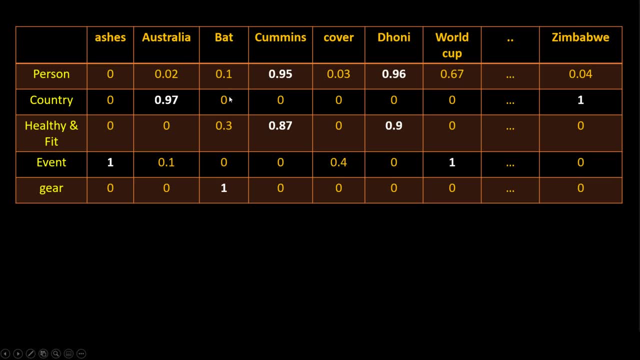 fit event gear, and when you have words like that, well, it's gear, so it's one. is it healthy and fit? you know, like when you train machine learning model, you might come up with these random numbers. so but overall you get an idea that if it is Australia country, then 0.97. 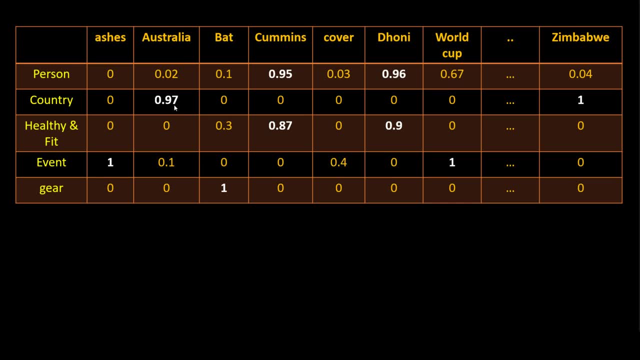 one means it's perfect. 0.97. yes, it's like like country. so again, I'm not putting one here, but showing 0.97 as an example, because these features, by the way, are not handcrafted here. I handcrafted this feature, but we will be using machine learning model later. 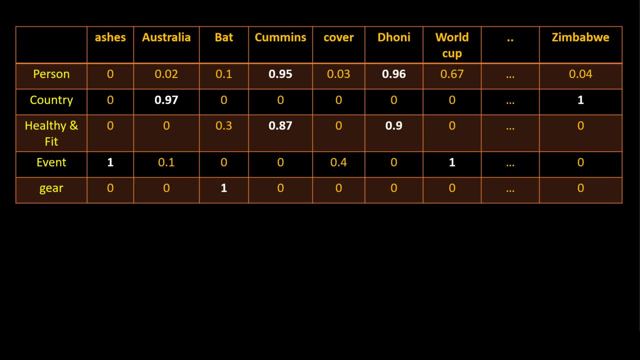 to come up with these features and you wouldn't even know what these features are, and it will just magically work. I will cover more that of that in future, but for now just assume there is some magical way of retrieving features from the words when you process a large corpus of text data. 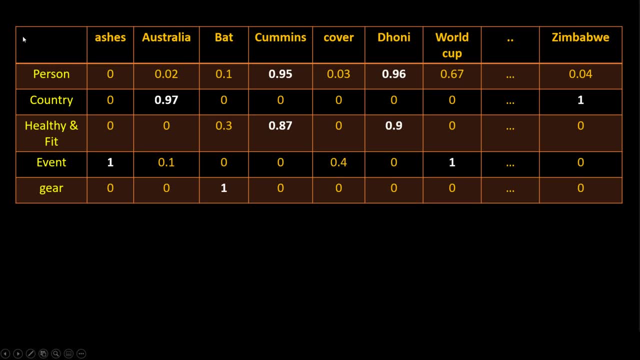 using using machine learning. so using machine learning, you can derive this kind of feature vector. okay, and once you have that, of course, when you look at features for Cummins versus Dhoni, they are matching, so you know that these are, these two are players. and when you look at feature vectors,